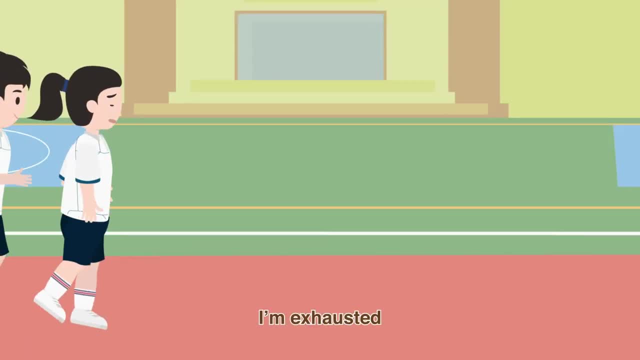 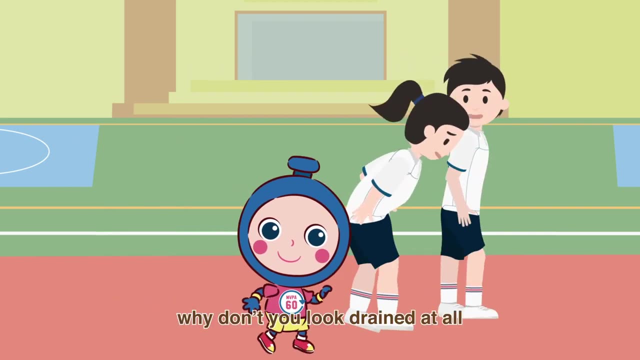 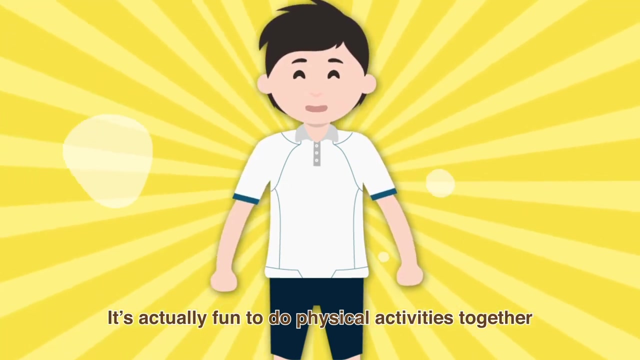 I'm exhausted. I can't feel my legs anymore. Keep it up, Sufa. Let's cross the finishing line together. Why don't you look drained at all And you seem to enjoy running so much? It's actually fun to do physical activities together and it's good for our health too. 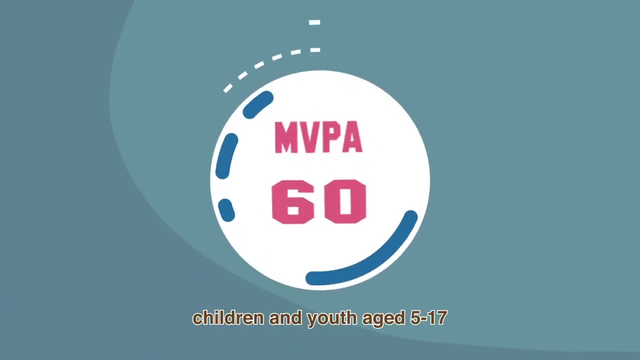 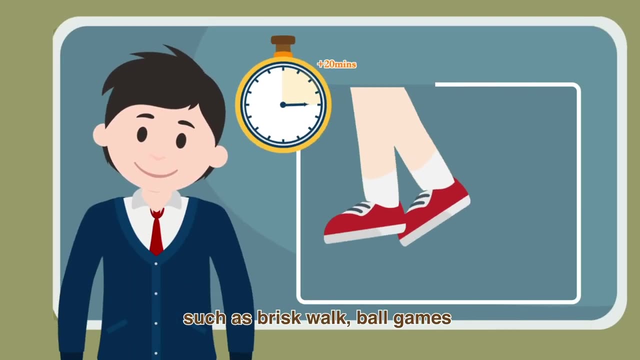 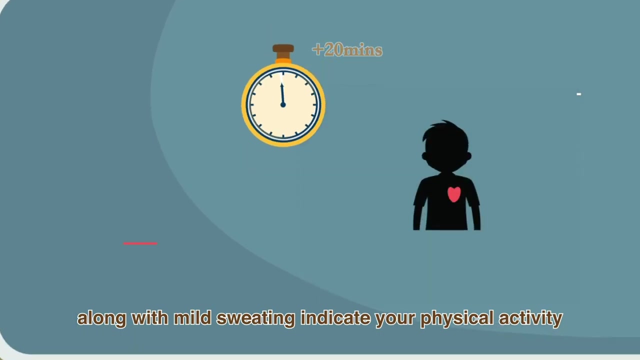 The World Health Organization recommended that children and youth aged 5 to 17 should accumulate at least 60 minutes of moderate to vigorous physical activity, such as brisk walk, ball games or walking up and down the stairs every day. Slightly increased breathing and heart rates, along with mild sweating. 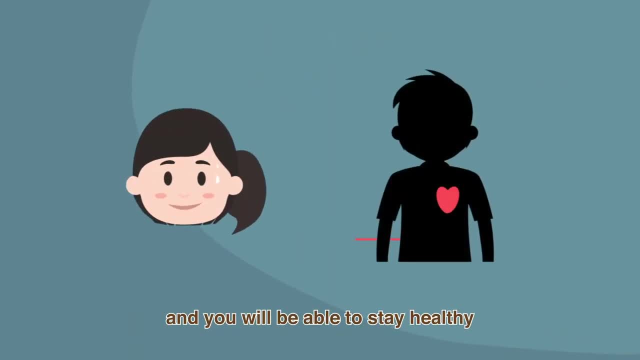 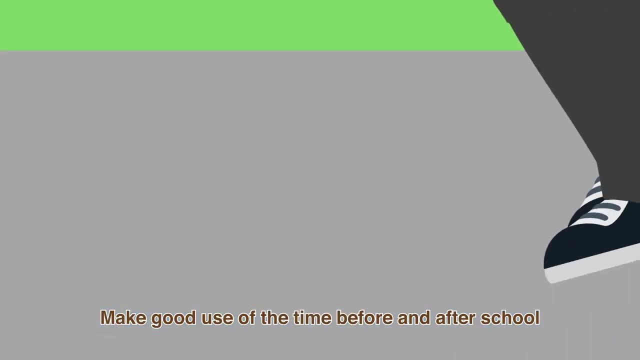 indicate your physical activity has reached the desired intensity and you will be able to stay healthy. It's not difficult at all to reach a cumulative 60 minutes of physical activity. Make good use of the time before and after school. You can walk briskly to school and back home under safe conditions. 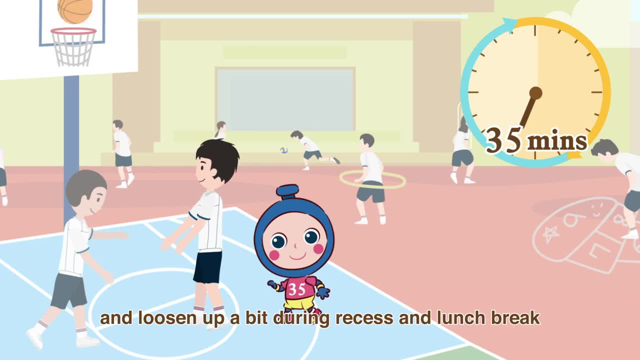 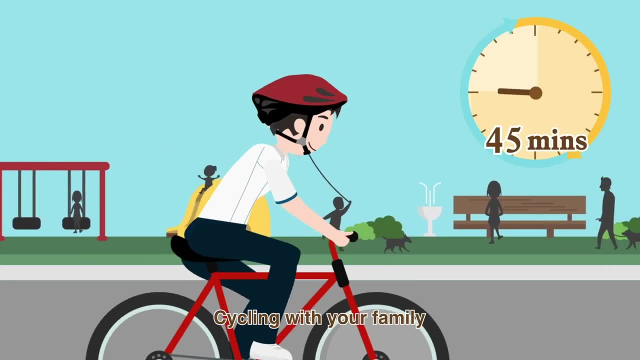 You can take part in different physical activities and loosen up a bit during recess and lunch break. How about with chores? when you get home? Sweeping and mopping the floor are also good physical activities for us, Cycling with your family or taking a walk with them. 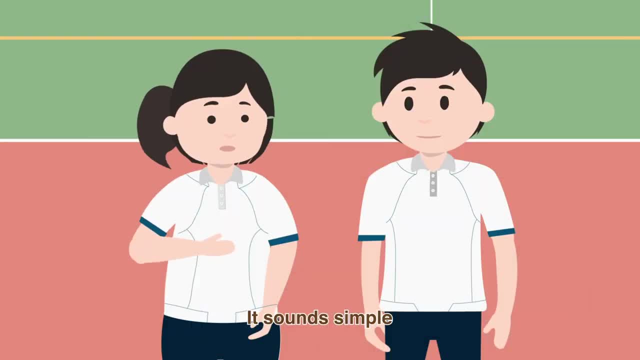 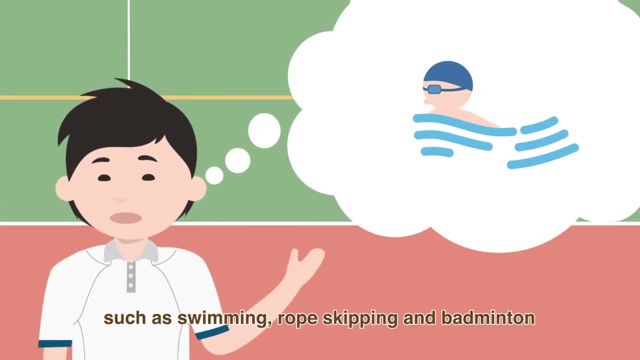 As a result, you have reached the 60-minute mark. It sounds simple. What physical activities do you like? Besides brisk, walk and playing in the park, I also play sports such as swimming, rope skipping and badminton. There are many kinds of physical activities. 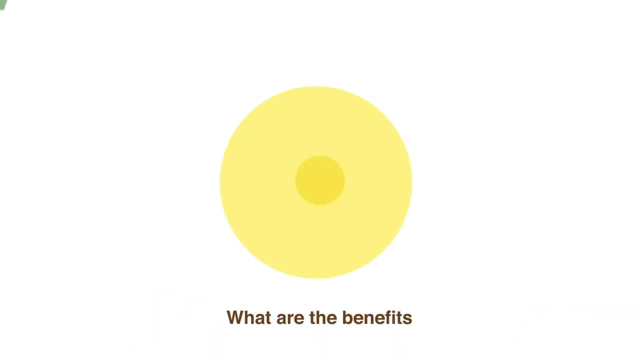 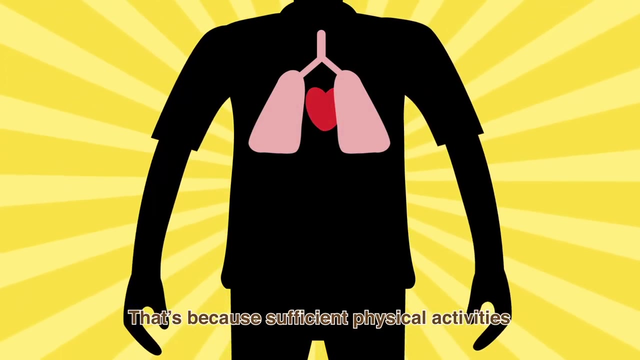 You can easily find one that best suits you. What are the benefits of doing regular physical activities? There are many benefits. Look at me, I don't get out of breath easily. That's because sufficient physical activities help boost your cardiorespiratory endurance, as well as strengthen muscles. 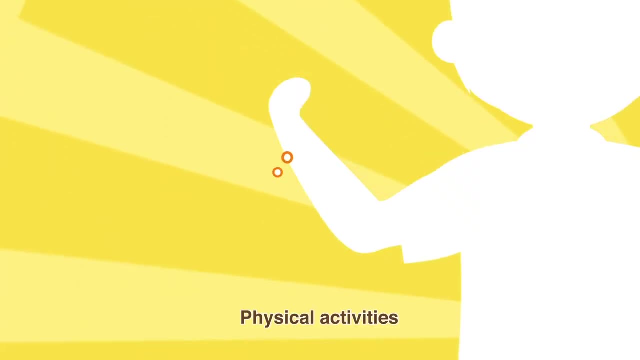 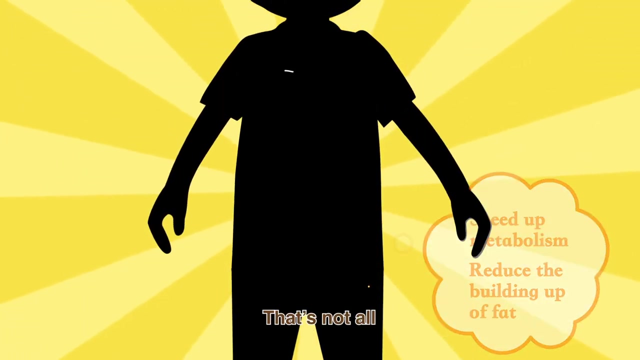 It even lowers the risk of cardiovascular disease. Physical activities also keep your muscles and bones healthy, speed up metabolism and reduce the building up of fat. That's not all: Doing exercise can help relieve anxiety and depression. It even has a positive impact on study goals. 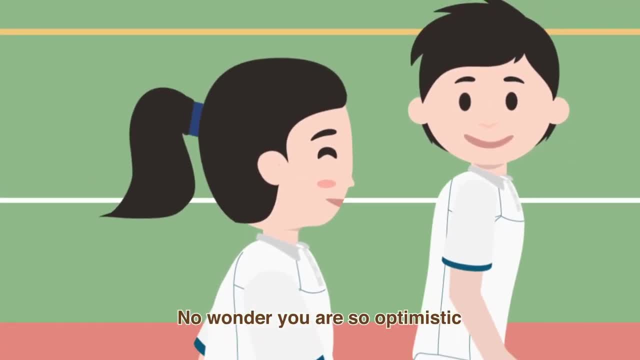 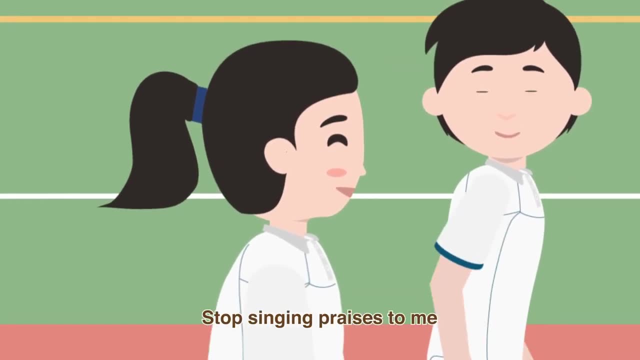 Does your body not feel lost and stressed? By doing exercise you will increase every kind of warm-up and okayness and financial stability. If you use exercise regularly, you will have a healthy diet. In fact, if you don't exercise, you're Coordinator Angel.